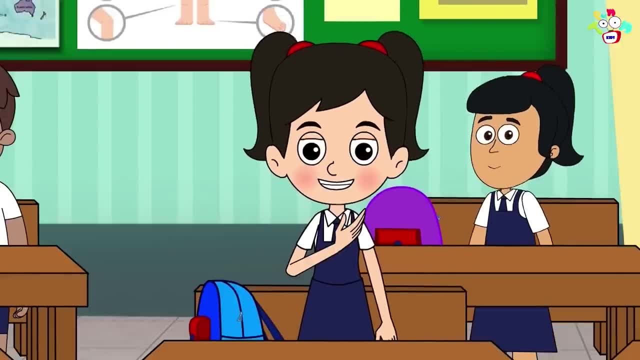 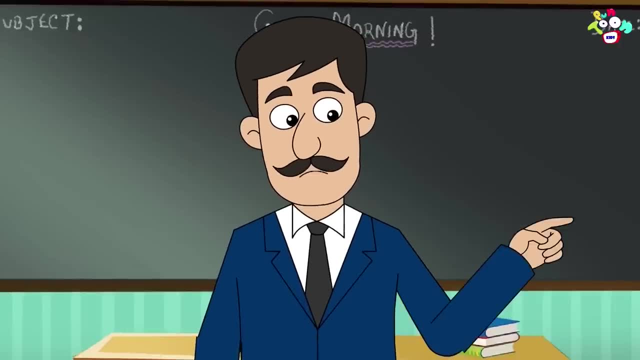 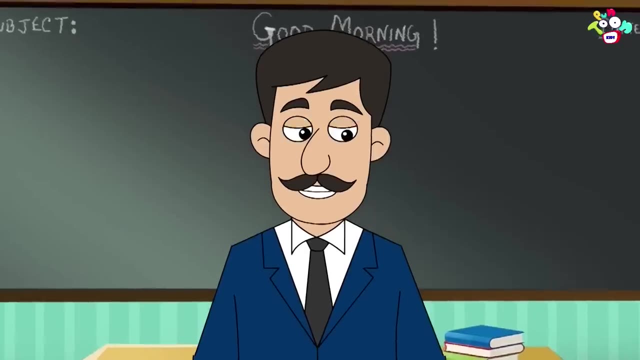 Next: Hello sir, I am Chinky and I love painting Beautiful. Yes, kiddo, So what is your favourite subject? This question was for Gattu. When Gattu stood up to answer, then the whole class, along with officers' attention, was on Gattu. 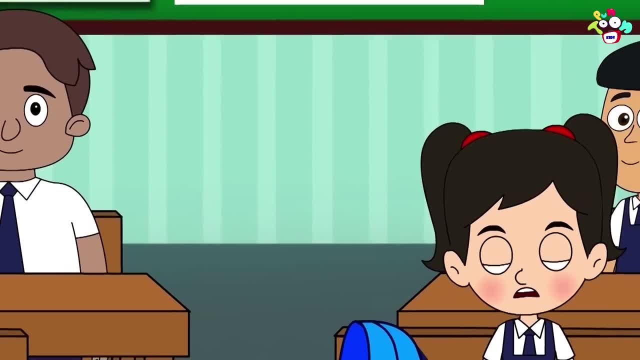 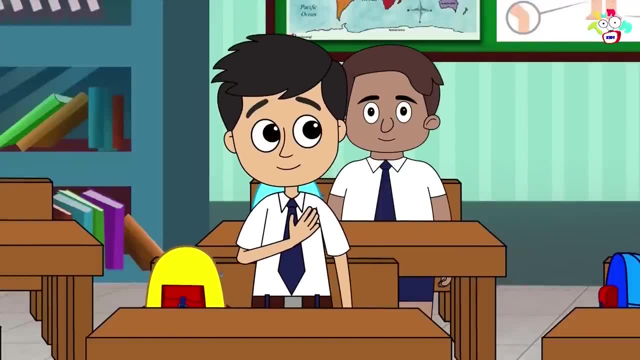 Now, which subject will Gattu choose? And as soon as Gattu told the name of the subject, everyone was shocked. Hi sir, My name is Gattu and my favourite subject is Maths. Oh, very impressive. Then Bunty meddled and said: 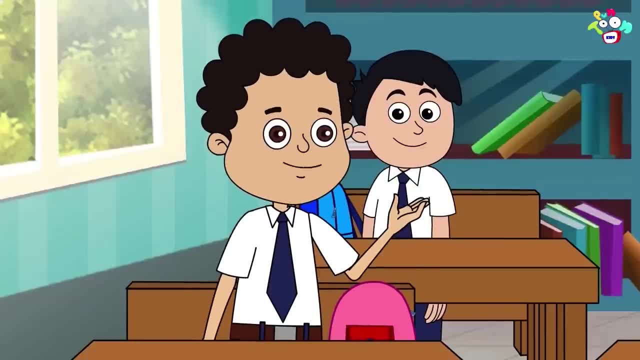 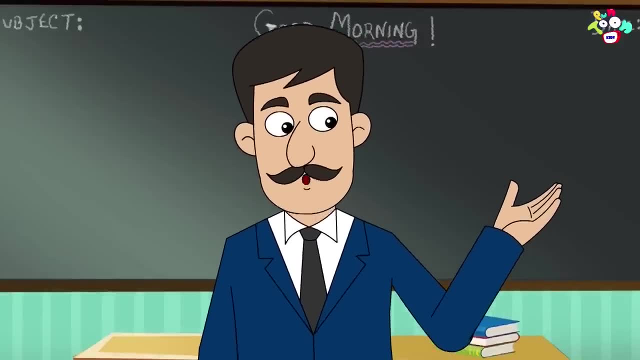 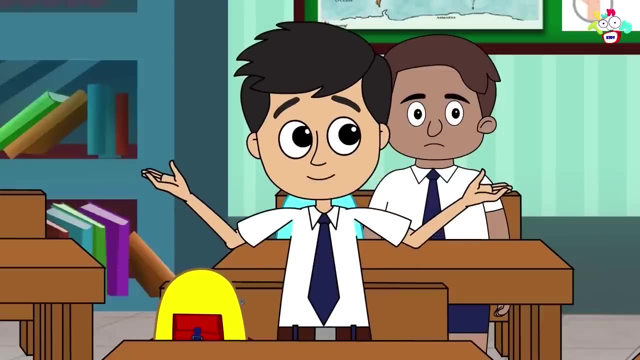 Sir Gattu is lying. He likes Science, not Maths. Gattu, whatever Bunty is saying, is it true? It was true till yesterday, sir, But today it's not. I used to like Science till yesterday, But today I like Maths the most. 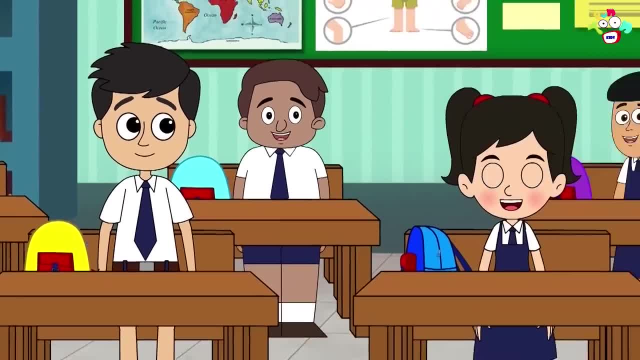 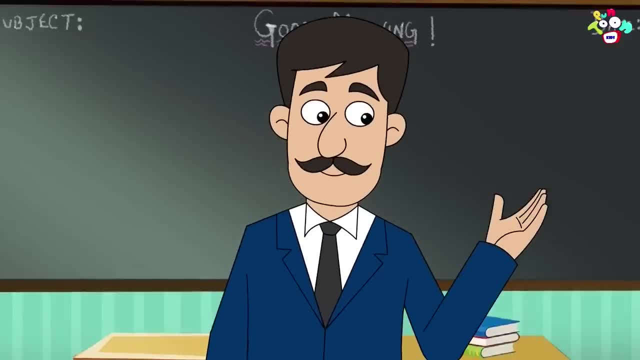 Hearing this answer of Gattu, the whole class started laughing. Oh, Gattu, Saying isn't enough, You have to show it through your actions. Nice idea, Bunty Gattu. if you really like Maths, then I will give you a numerical problem on the board. Solve it and show it. 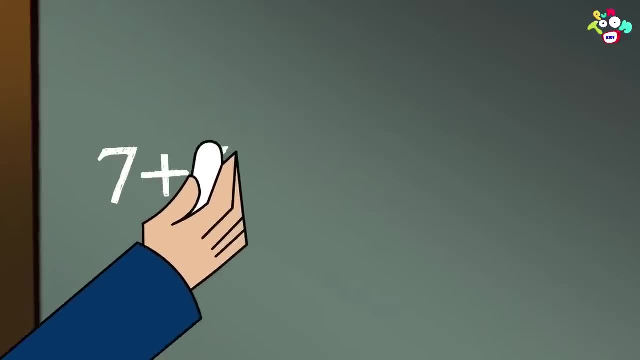 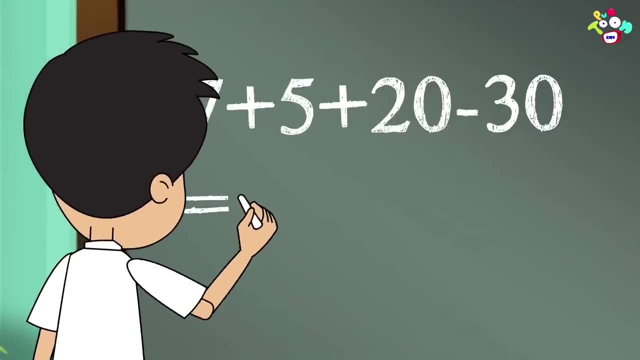 Now it will be fun. Then the officer wrote a numerical for Gattu on the board and asked him to solve it. Gattu came to the board and solved that numerical problem in a jiffy. Excellent, All of you please clap for Gattu. 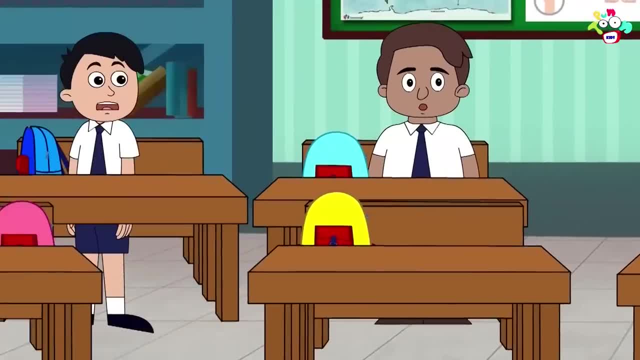 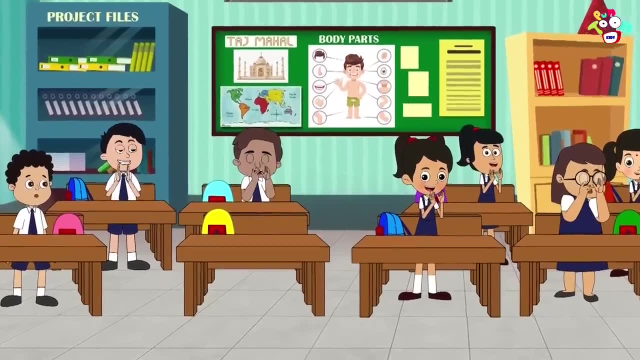 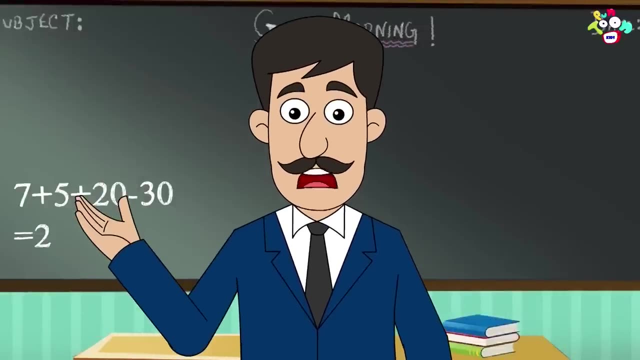 Everyone was shocked to see Gattu's confidence and performance. Bunty could not understand how all this happened. The whole class felicitated Gattu with applause. Most of the children's favourite subjects are English or Art subjects. Many children are also afraid of Maths. 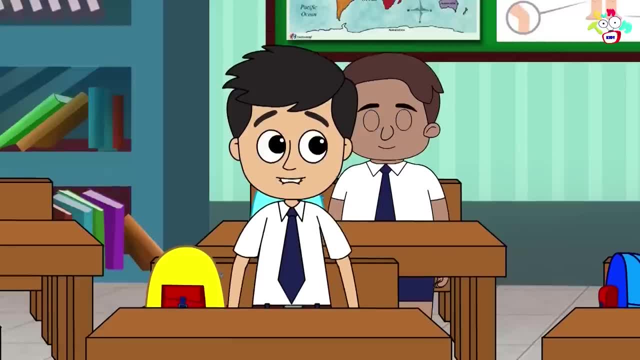 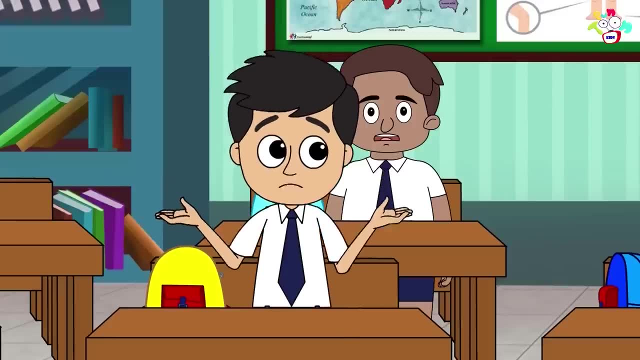 Tell me, Gattu, why do you like Maths so much? Because, sir, Maths consists of numbers and I enjoy playing with numbers. I talk to the numbers, They also talk to me, And by just talking like this, questions get solved. 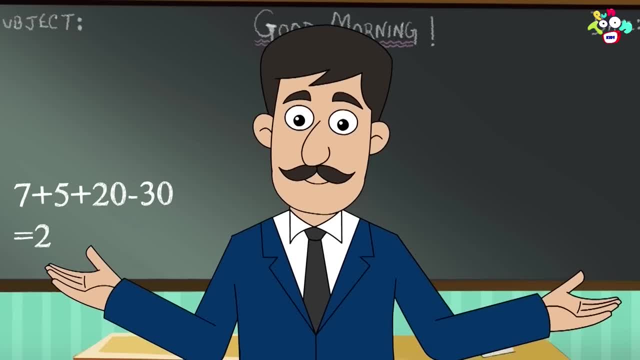 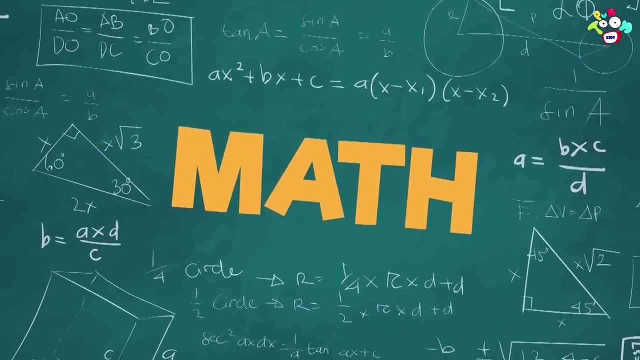 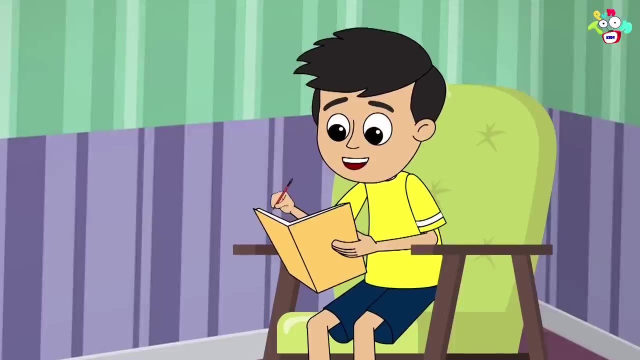 Oh, how interesting. So now you all know, our Gattu's favourite subject is Maths. Is Maths your favourite subject too? Talking about Gattu, Gattu's Maths love was not limited to just class and notebook. Maths used to stay with him at his place. 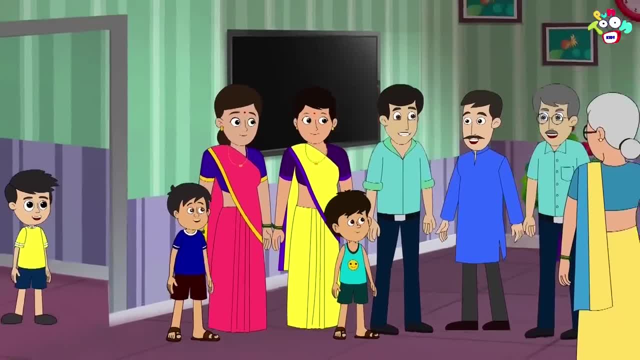 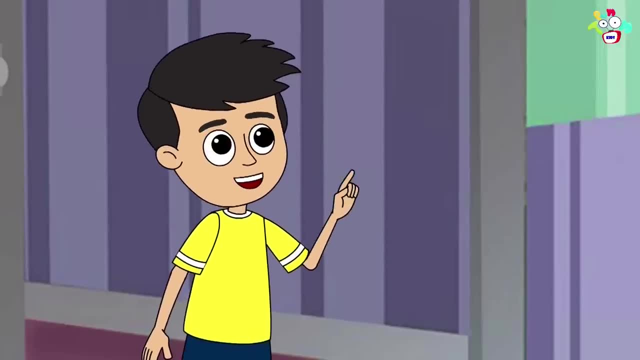 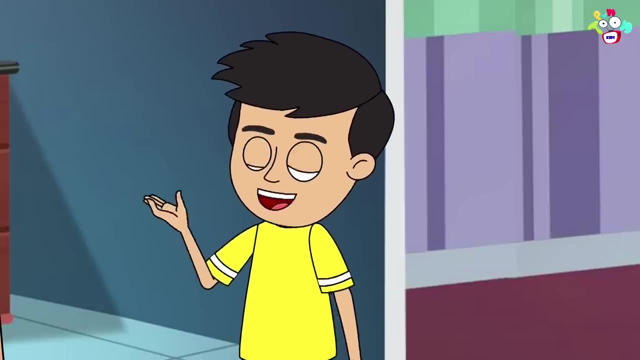 One day there were many guests in the house. Gattu silently counted all the guests: 1, 2, 3, 4. Gattu ran towards the kitchen and told his mom. Mom, there are total 14 people, 4 of them are small children, 6 young and the rest 4 are old, around grandma's age. 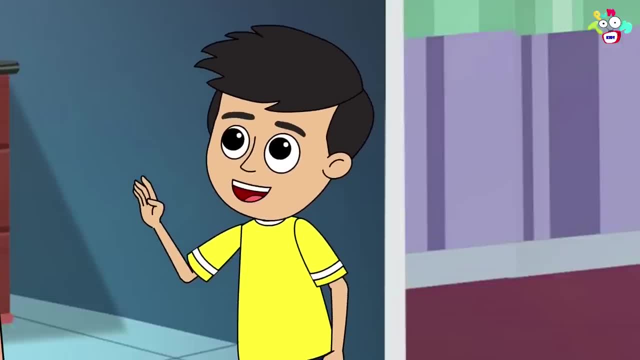 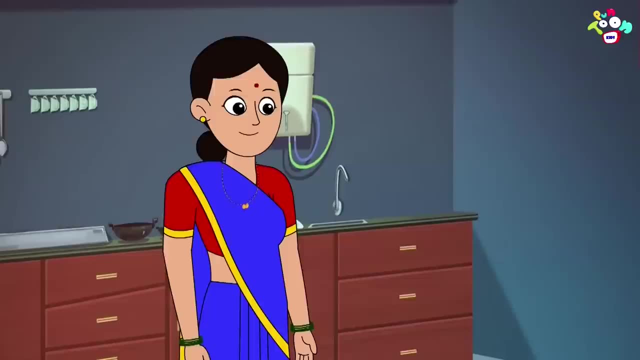 That means you can prepare 4 glasses of milk for the children, 6 mugs of coffee for the young people and 4 cups of tea for old people. Hearing Gattu's statistics and logic, his mother went blank for a few seconds. 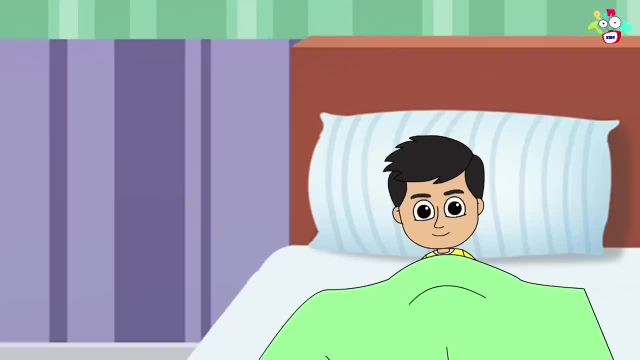 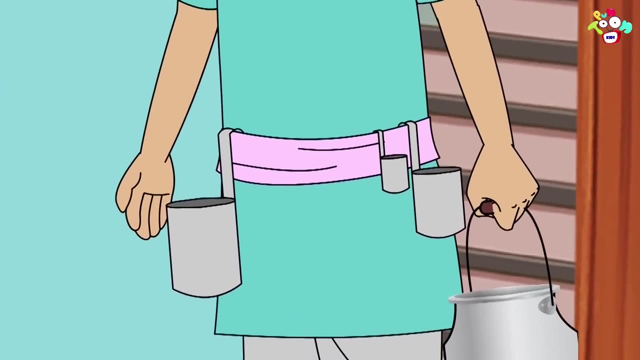 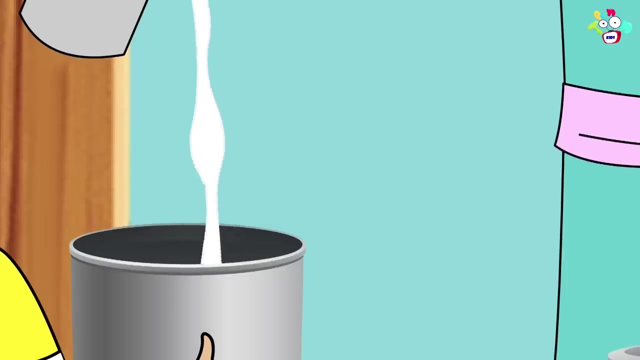 Whenever the milkman used to come, Gattu would get up every morning to take milk. The milkman had small aluminium measuring cans of 1 litre, half a litre, by which he used to pour milk into the pot. This is 1 litre, this is half litre, and here is your 1 and a half litre, Gattu. 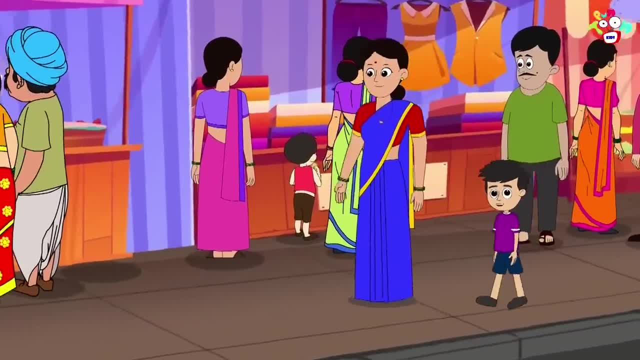 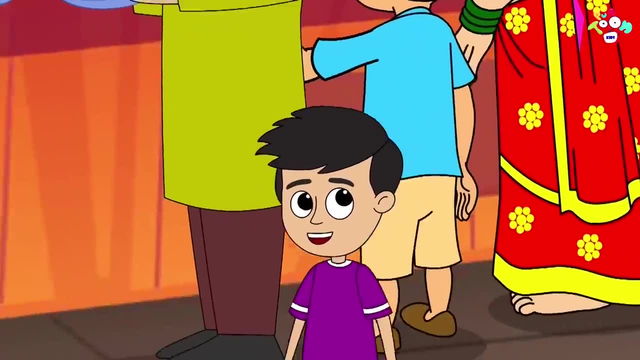 Gattu used to go to the market with his mother. Even then also, Maths did not leave him. While buying vegetables from the vegetable seller, Gattu's focus used to be on the money, But the vegetable vendor was more perfect than Gattu in Maths. 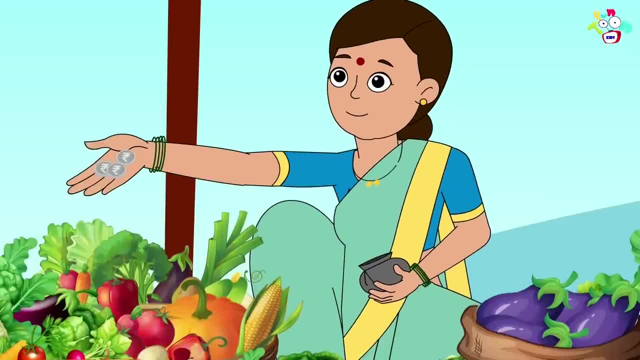 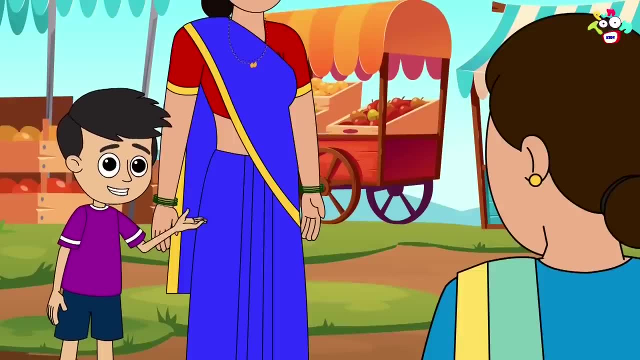 As soon as she used to give a note, she quickly used to take out the money and give the remaining money to her mother, and that amount was absolutely correct. Aunty, you don't have a calculator Yet how do you calculate so fast? 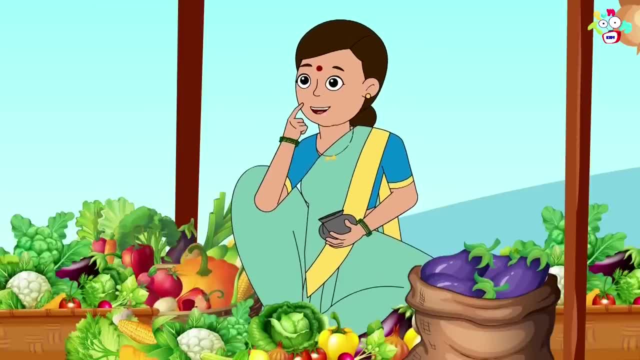 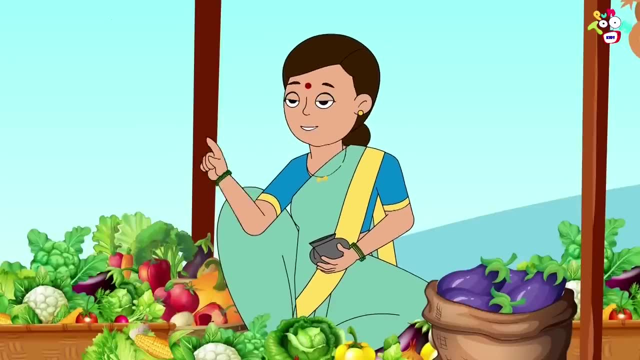 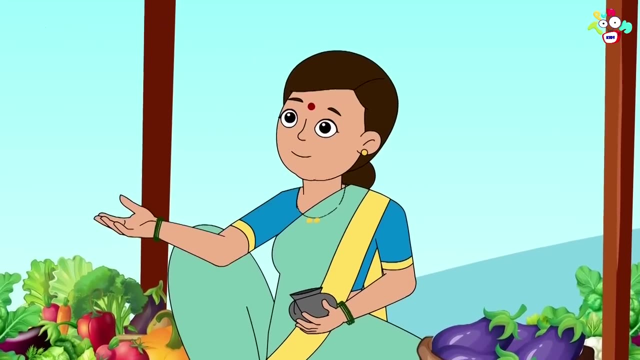 Son, I know how. What do they say in your language? Umm, Experience, Yes, Experience. I learnt from experience. Initially, I used to make a lot of mistakes. Used to give more money to some customers, then less to some.